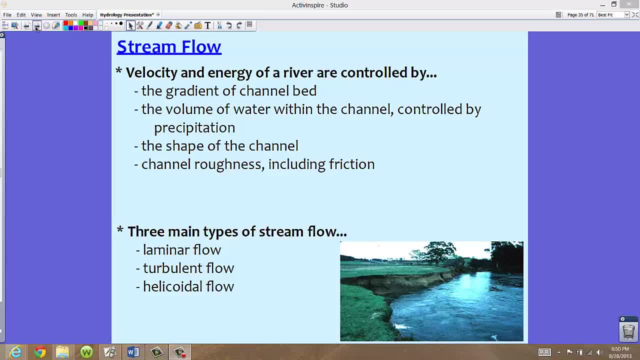 some of them might be a little bit more like diagonal. It depends on the shape of the channel And channel roughness, which includes friction. So the channel roughness depends on how large particles your big boulders versus just sand or clay. 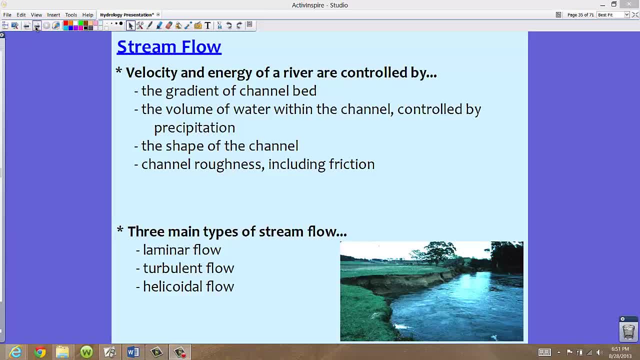 that might be in here. So the velocity of the energy of the river are controlled by those factors and the flow of the stream is controlled by those factors. Now, there's three main types of stream flow and we're going to talk about each of them in turn. 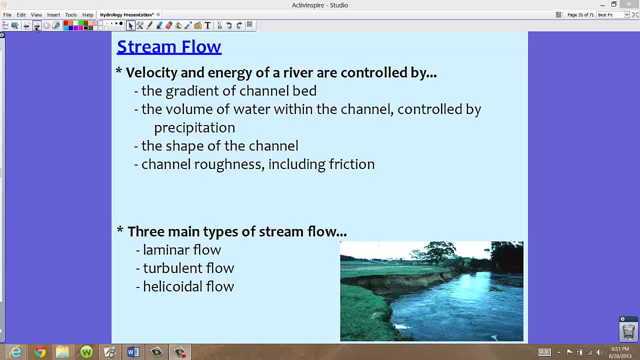 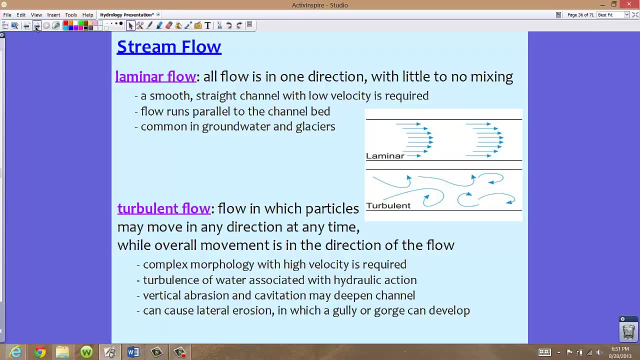 So we have laminar flow, we have turbulent flow and helicoidal flow. Now, each of them does something a little bit different for the land. So let's take a look. First, laminar flow. Now, laminar flow is all the flow in a stream. 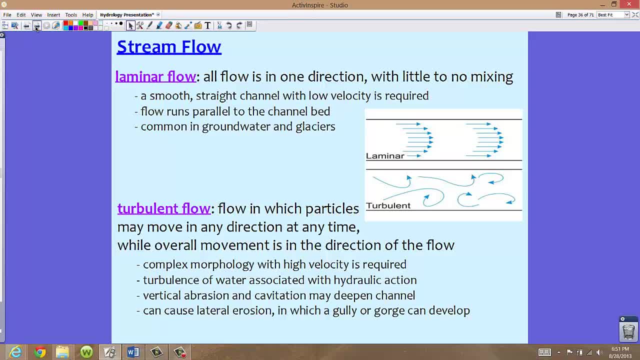 goes in one direction with little to no mixing. So all the stream, basically all the water, rushes directly in one way And that's it Now, unfortunately, this is not very common on surface waters, because we have a lot going on. So what we really need 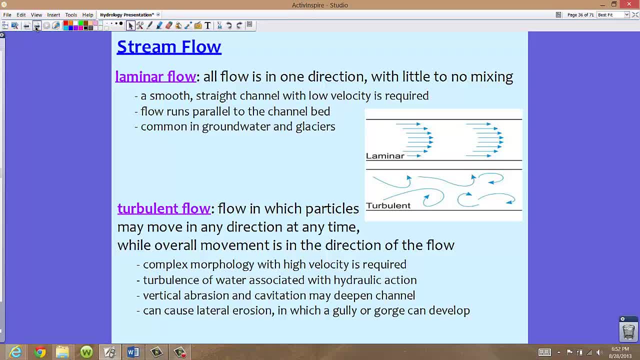 is a smooth, straight channel where there's a low velocity. Now this is a must if we are to see laminar flow. Typically, we see this a lot in groundwater or glaciers, So as glaciers melt, we see this Going in one direction. 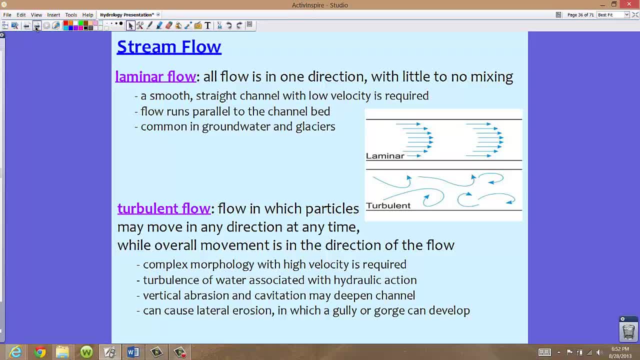 In groundwater. if we were to take a look, if we had access to look at groundwater, we would see that this also flows in one direction. Now the flow will run parallel to the channel bed, So all the water is moving in one direction. 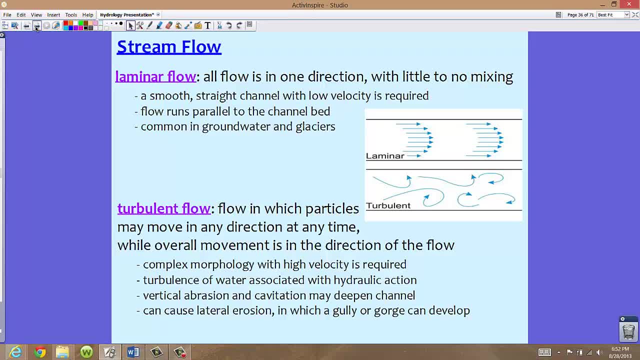 None of that water starts to go from side to side. it's directly forward, Directly in a straight line. So in this picture, notice the laminar flow. you can kind of see all of it just going in one direction. It's usually with the current. 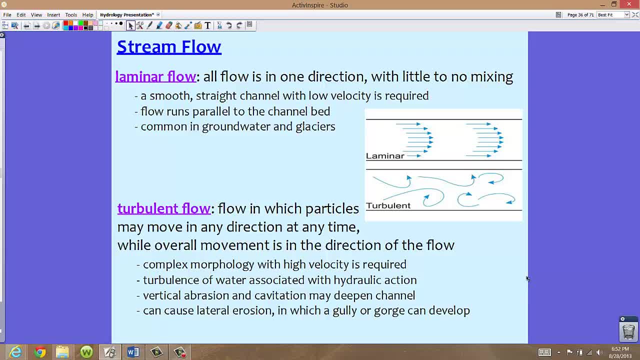 Our second type of stream flow is called turbulent flow. Now, this is the flow where the particles can move in any direction and at any time. However, the overall movement is kind of with the current, So it does flow in one direction, However. 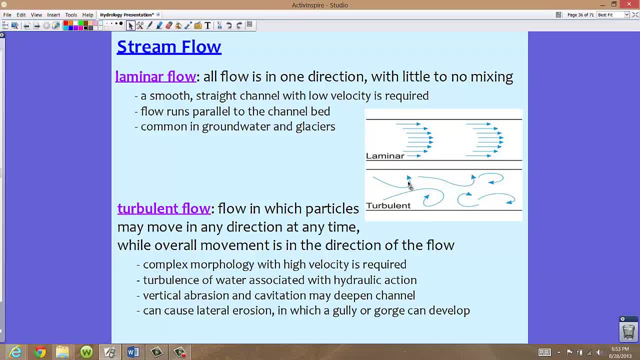 like you can see in the picture, it sort of moves in general directions. So you see a lot of the water, maybe kind of turning. It'll go down, it'll go under, create little circles. It's a very turbulent flow. Now we don't necessarily 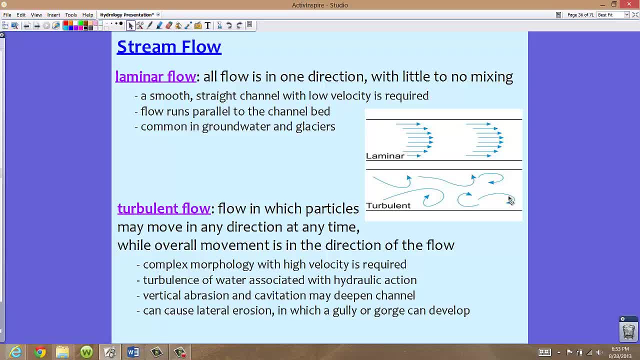 have to have a lot like a large turbulence in order for this to happen. It happens on normal streams most of the time Because, if you think about it, there might be big rocks in the way, there might be something in the way that requires the water. 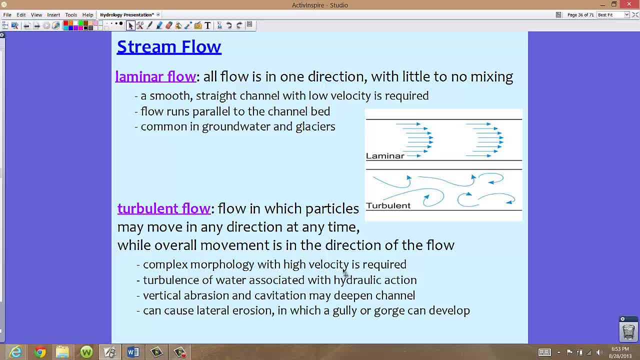 to sort of move around it, So complex morphology with high velocities required, So we do have to have a pretty high stream flow in order for this to happen. But you can sort of see this in some other places as well, like small streams that maybe don't. 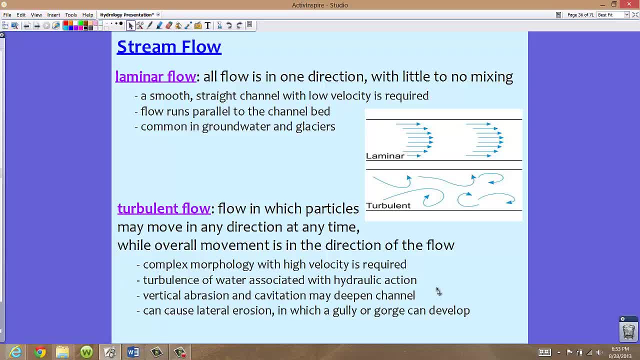 necessarily have a very high velocity. The turbulence of the water is associated with hydraulic action. Remember, in the last video we talked about that hydraulic action and how it causes basically air and water sort of get into those little cracks and they force those little cracks open. 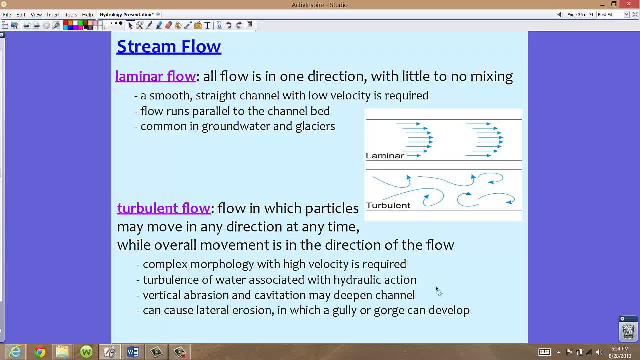 And that causes the erosion in those particular places. So we see a lot of hydraulic action in these types of flows. Now we also see vertical abrasion and cavitation which may deepen the channel. So vertical abrasion- remember abrasion- is basically. 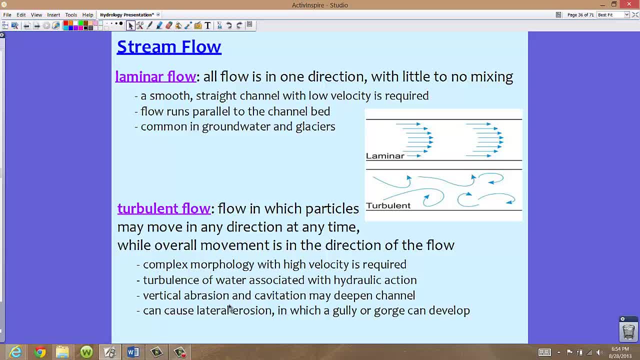 where you have those rocks and stuff eroding along the bottom, the channel bed and the banks of the river as well. So if it goes vertically, it means it's going up and down And it's going to deepen those channels. Cavitation also happens that way. 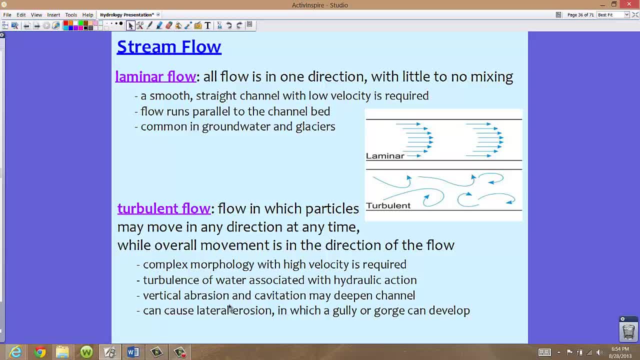 You see those little bubbles, those pockets of implosion, basically, and that's going to break those rocks apart And it's going to deepen that channel. Now, this could cause lateral erosion as well, And this causes a gully or a gorge to develop. 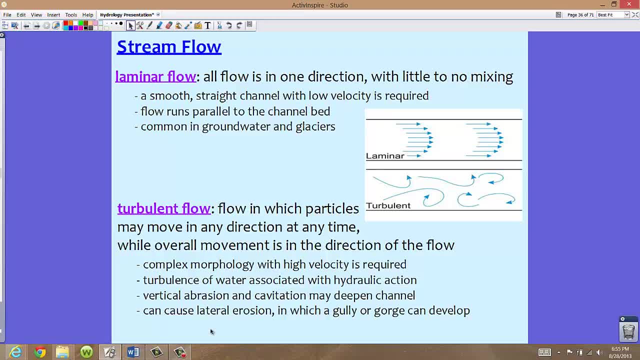 So if the banks are basically eroded away from side to side- and that's the lateral erosion, it's widening of the river And we might get a gully or possibly a gorge. So the Grand Canyon was actually formed in this manner, by turbulent flow. 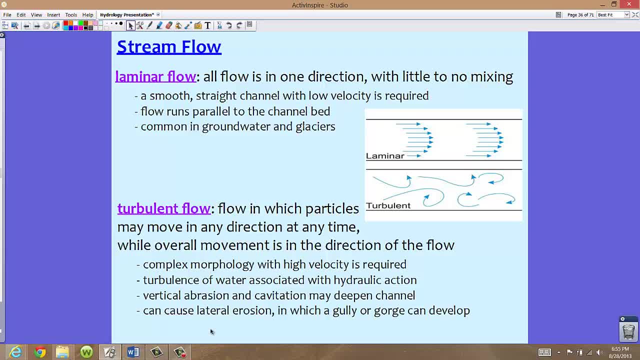 So the Grand Canyon is an excellent example of turbulent flow, especially by this vertical abrasion, and the cavitation, And sometimes also some of that lateral erosion has eroded away parts of the Grand Canyon. It's widened it in certain areas too. 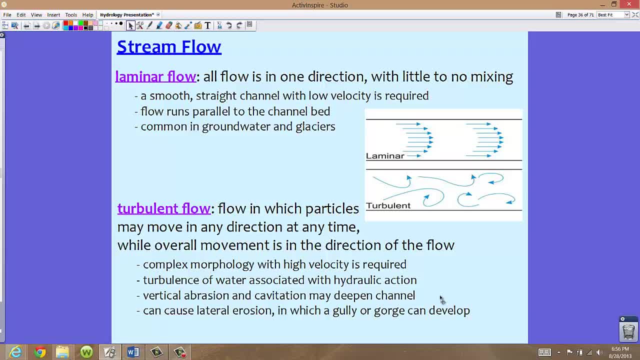 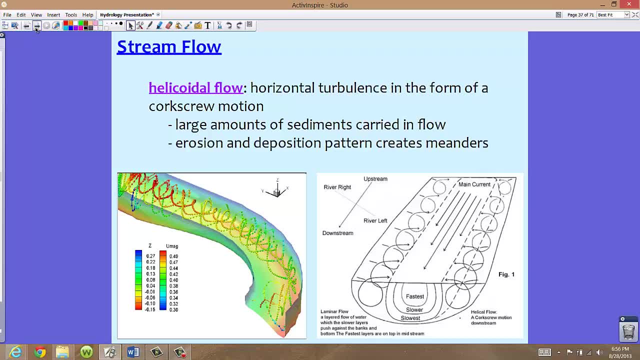 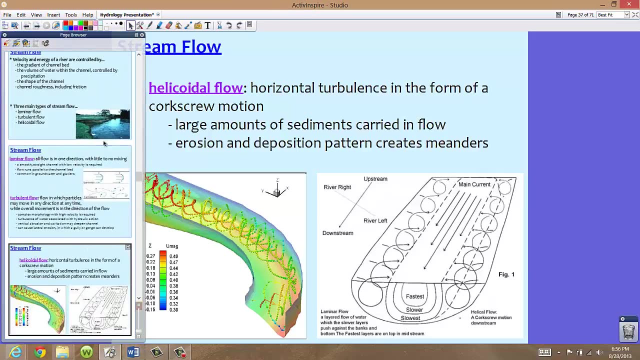 So with turbulent flow- think of the Grand Canyon. when thinking of an example- We also see helicoidal flow. Now, helicoidal flow is a little bit different because we see things, those water molecules are actually moving in corkscrew motions. 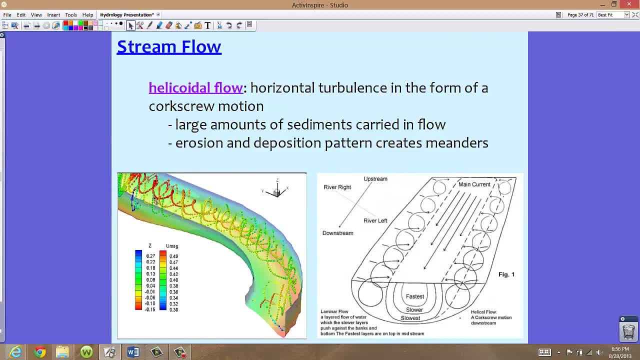 Oops, sorry about that. So in corkscrew motions, kind of think of that movement, kind of like a corkscrew up and down, up and down, You're going to have all these particles move that way In places like this. 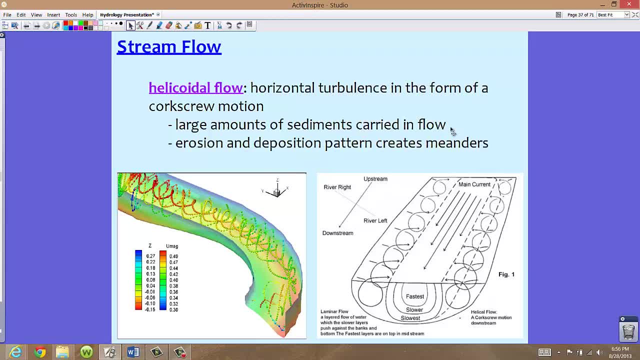 we actually see large amounts of sediments carried in flows like this, And this creates meanders, And soon we're going to be talking about meanders, But if you think of somebody meandering back and forth, back and forth, helicoidal flow works the same way. 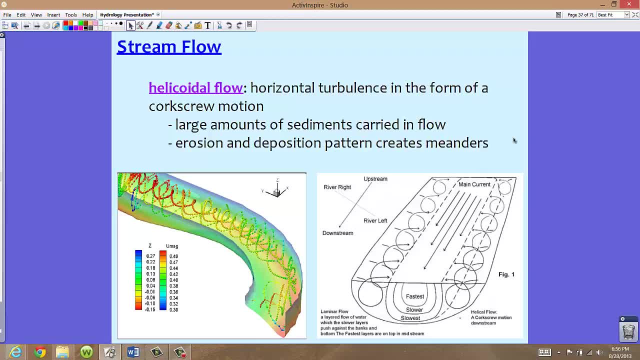 We have this corkscrew motion of the water molecules and it's creating the water to kind of go back and forth and eventually it creates those large meanders that are so prevalent in some areas. So in this picture we see more of a 3D model of it. 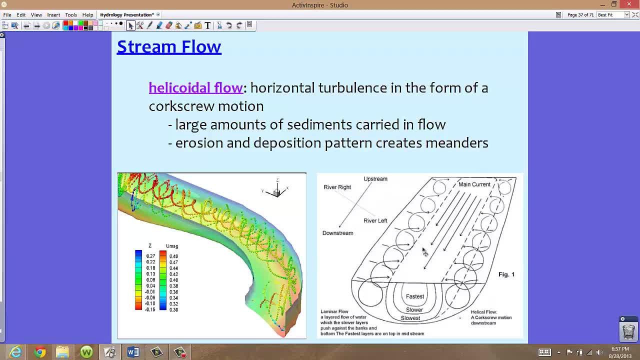 or what should have been a 3D model, Whereas the right hand side, this figure one, we can kind of see the corkscrew motion kind of doing this with the main current, kind of still going down the middle. But that corkscrew motion really messes. 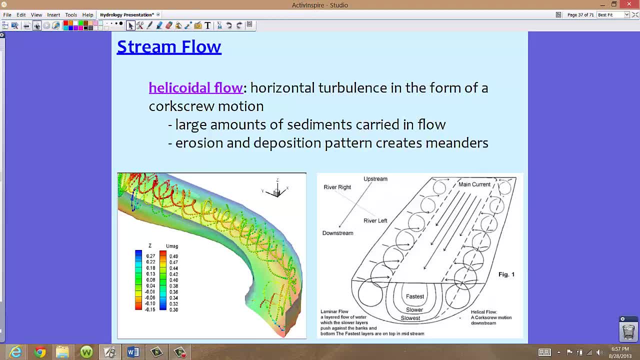 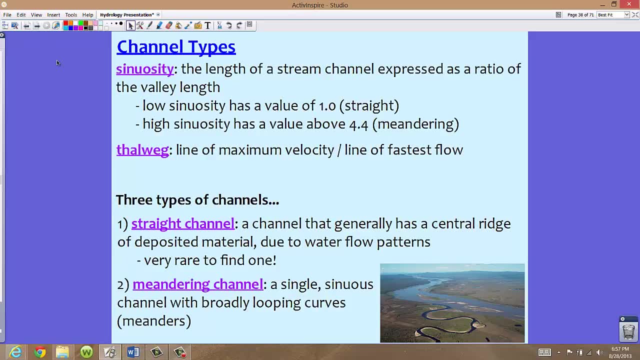 with a lot of that side-to-side movement of the actual channel. Now we see different channel types And this is all really because of these types of flows, So you can actually go back and sort of match up from one place to another. A couple words to sort of know. 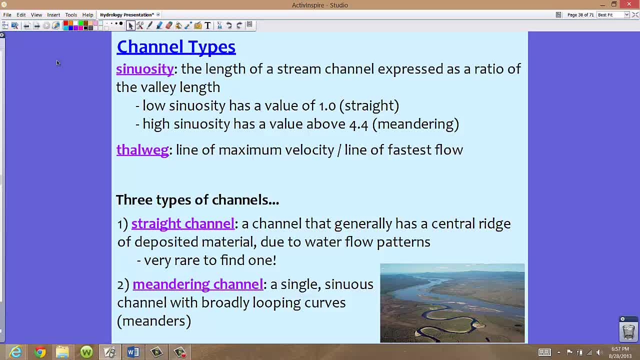 to throw more vocabulary at you: Sinuosity, Now, this is the length of a stream channel that's expressed as a ratio of the valley length. So it basically is talking about the valley length and we're putting a ratio to it on how 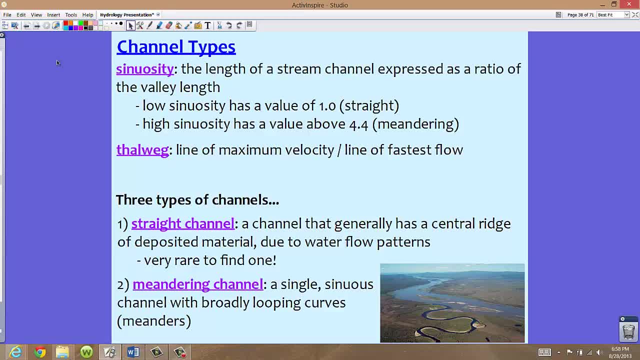 long the stream channel is How long the channel actually is. So we're said to have- or a river is said to have- a low sinuosity, Typically if it's a straight channel, And we're going to talk about what a straight channel is. 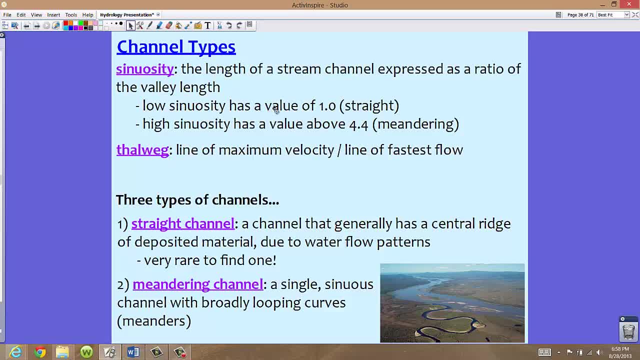 So anything that has a value of about one or close to one in that very general area has a low sinuosity. Anything that has a high sinuosity is said to be above 4.4, and this is going to be meandering. 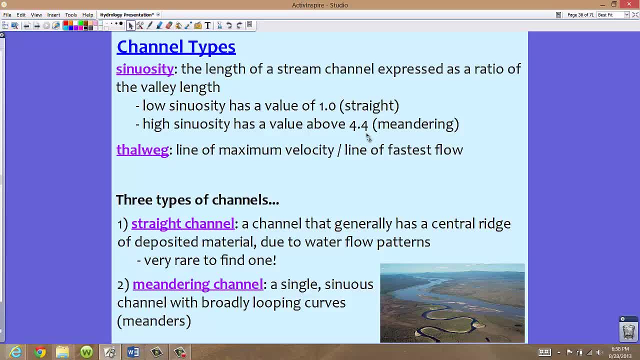 So if you take the length of the channel, it might be longer than the valley length that it runs through. So this is why meandering rivers, as the picture down here kind of shows, these are going to be technically longer because there's more river. 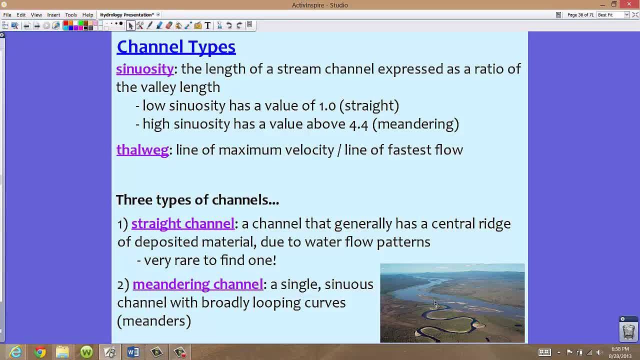 There's more channel, Whereas if it was a straight channel, that'd be pretty low. The ratio would be pretty close to one to one. Now we also see this term, thalweg, And this is the line of maximum velocity, or basically the line. 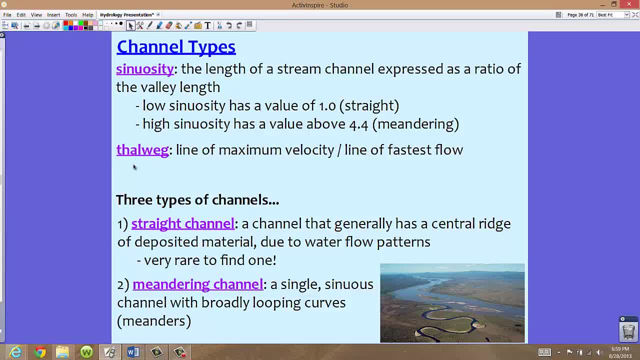 of fastest flow. So in some cases, and so far, we're really not going to talk too much about thalweg, but in some cases along the river there are some geologists that actually go through and they test a certain length of river. 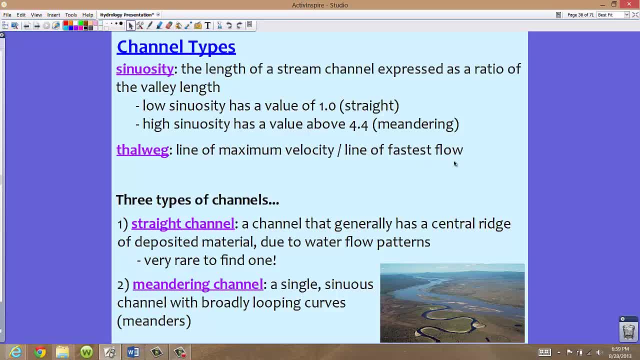 to see where that line of fastest flow is, Because the flow changes along the river, So it's very important to know where exactly that line is along the river. And people do that And that's called the thalweg- How fast a certain point is going along the river. 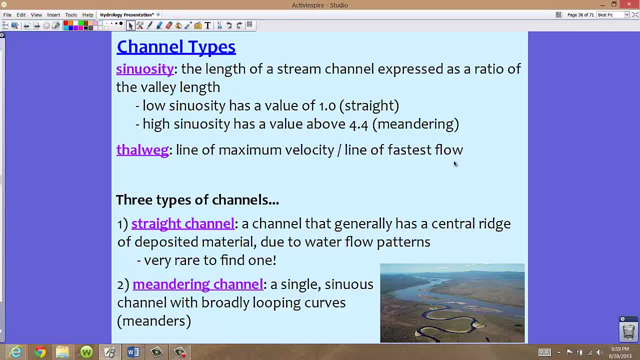 The fastest point. there. There are groups of channels and I sort of mentioned two of them. up top We have a straight channel. Now this channel is generally has a central ridge of deposited material, So on the sides we have some deposited material. 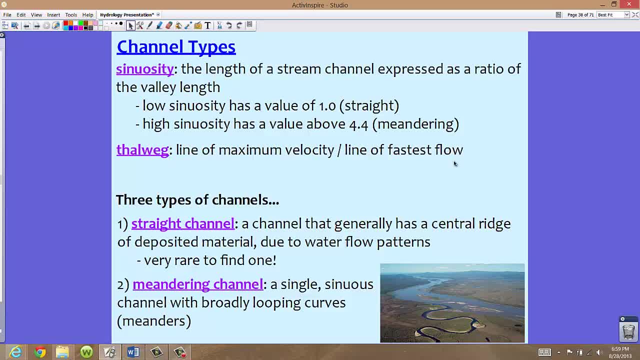 And that's because our water is just basically going straight. This is what you would see in laminar flow, Basically, where the water is going directly straight. These are really hard to find because they're by over time it's going to start to meander. 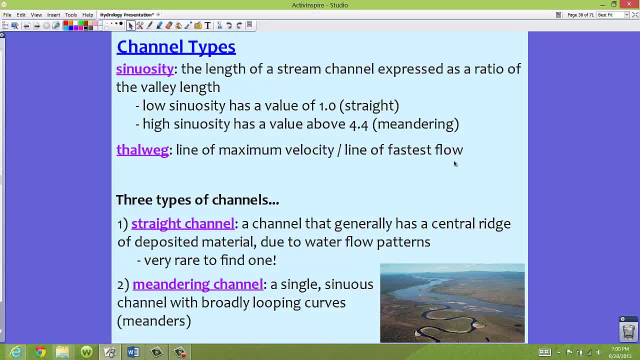 It's going to start doing that side to side motion. So straight channels are really hard to find. We see these a lot in young places, like very young rivers, or perhaps in areas like glacial areas, where we have just a nice steep gradient and we have a nice straight channel. 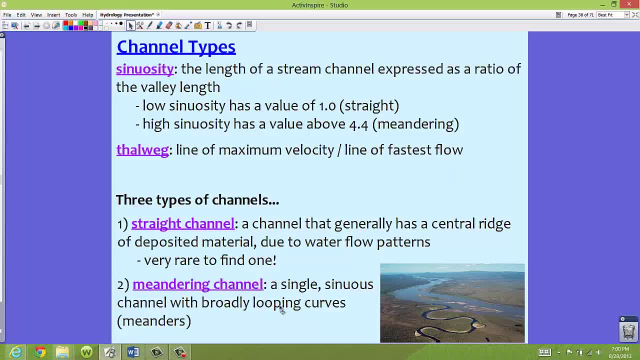 from there. A second type of channel is called the meandering channel, And this is where you get those long curves back and forth, And in the picture you can sort of see this nice meandering channel right here. So whoop, whoop, all that nice meandering channel. 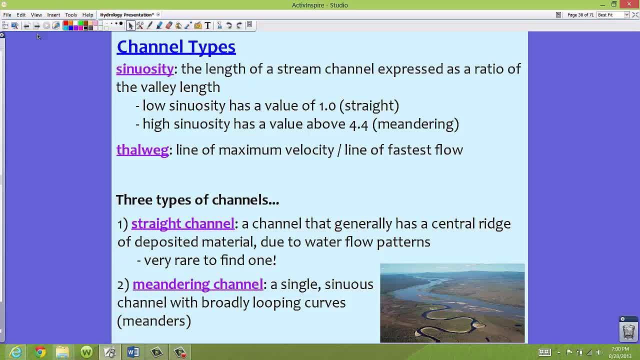 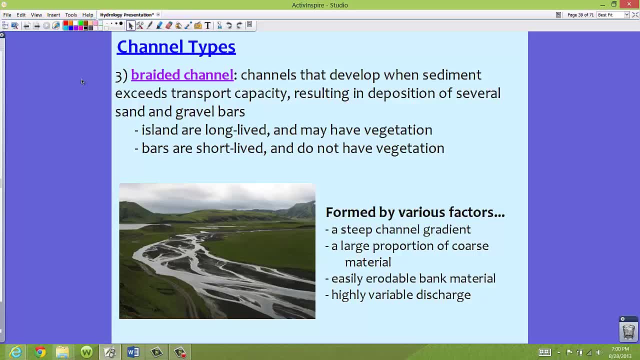 And that's going to form because of that helicoidal flow that we just talked about. We also see a third type, which is called a braided channel. Now, this is probably a little bit more seen in some places, partly a lot so much in Florida as well. 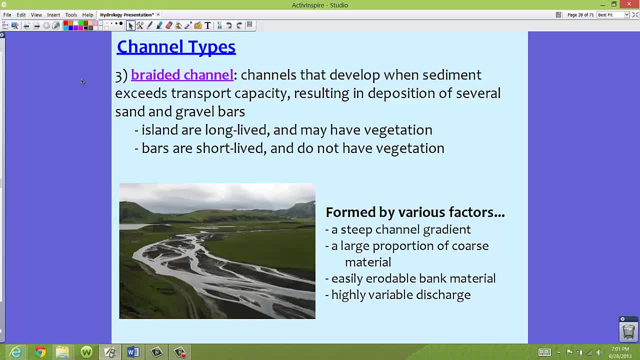 because of our level of water that we see in some channels. But these are channels that develop when sediment exceeds transport capacity, So there's too much sediment in the actual water. The water can't hold it all, So this results in deposition of several sandbars and gravel bars. 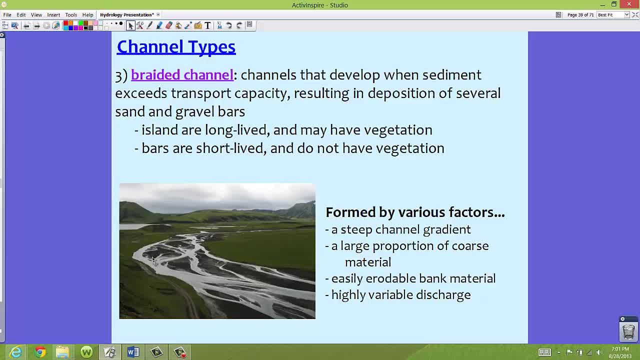 And so you can kind of see in here. you actually see all these places of sediment that were dropped out of the load. There's not enough water to carry all that sediment, so it's basically just deposited right there. Now, islands are long lived and they may have. 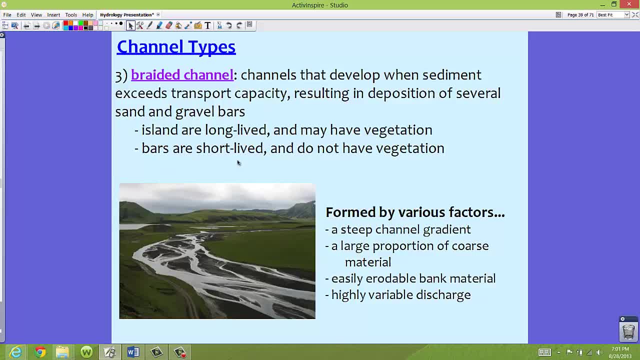 vegetation, Whereas bars are short lived and they do not have vegetation. So if you see a river kind of like this and there might be some vegetation growing in the middle of one of these islands, you know that that's been there a pretty long time. 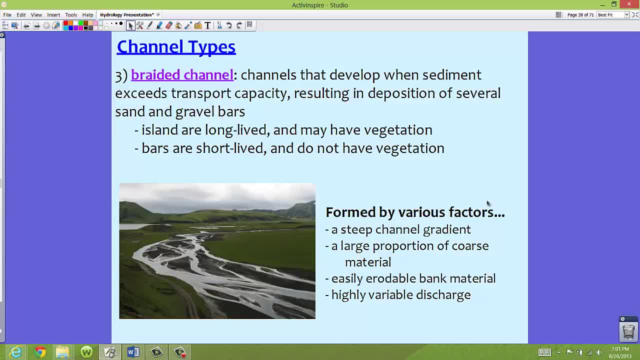 Now, these are formed by various factors as well. Perhaps we have a really steep channel gradient, Perhaps there's a large proportion of coarse material, Really large rocks, going on. Perhaps there's an easily erodible bank material along the side, Like in this. 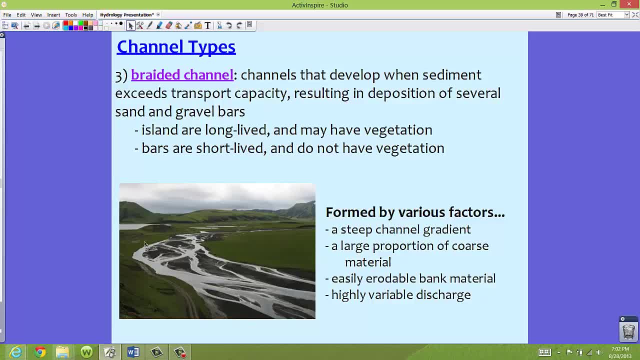 case, that's sort of what it looks like. This area is really nicely eroded So we can kind of pick it up. The water kind of picks it up as it goes, But it's not fast enough. There's not enough capacity in that river.